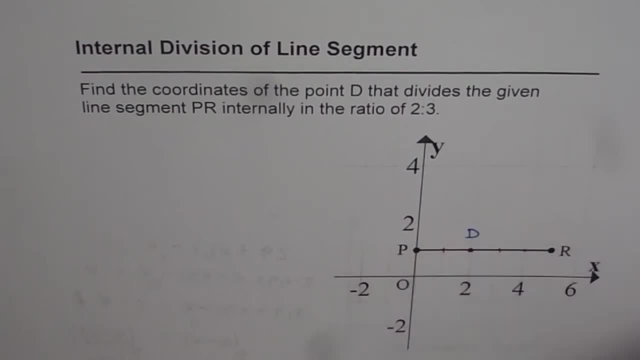 So let me write down point D And since we have a coordinate plane, we know D is 2, 1,, correct? That is the coordinate For point D. ratio 2 is 2, 1.. This P to D is 2 for us and D to R is 3, 1, 2, 3.. So D divides PR in the ratio of 2 to 3.. Simple, So we get our point in this particular case. 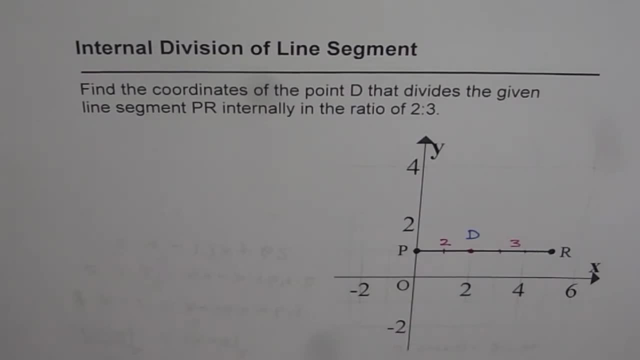 Now let's extend it to vectors and see how to find the coordinates of this point D, given points P and R. So in this case, if you see what are points P and R, Point P the coordinates are 0 and 1, correct. And for R, the coordinates are 5 and 1, correct. 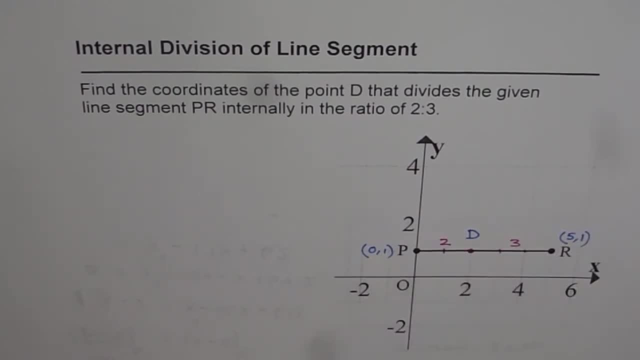 We need to find coordinates of points. So what we can do is we can treat external point O, which is the origin, and from here let's look into the position vectors: OP, OD and OR. Now, if I can relate OD with OP and OR, OP and OR are known to us. 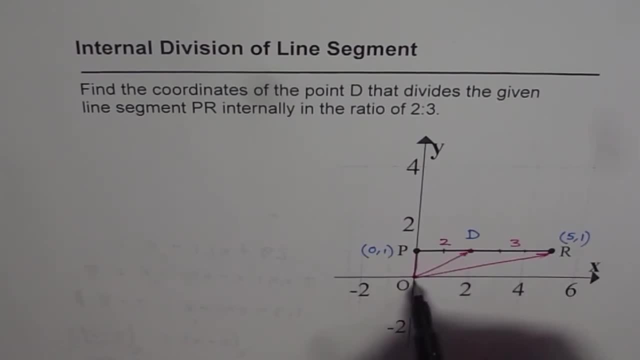 Then I can find OD. Once I get the position vector OD, then I know the coordinates of D also correct. So that is the strategy which we are going to use in vectors. Now let's work it out How to find relation between OD, OP and OR, So that becomes our problem now. 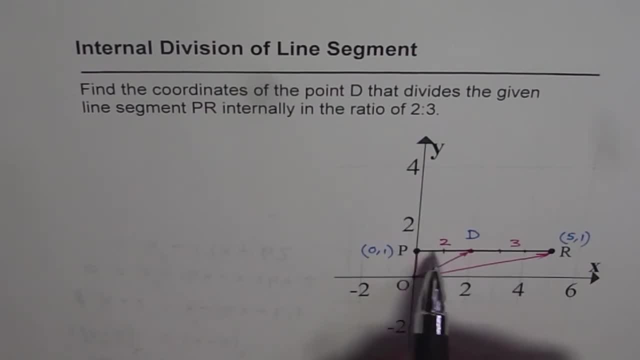 Let's start with saying what is relation of PD with PR. We can say: well, PD vector, PD law is collinear with PR. It's a scalar multiple right. So if I divide PR into 2 plus 3, 5 parts, then PD should be 2 parts, correct. 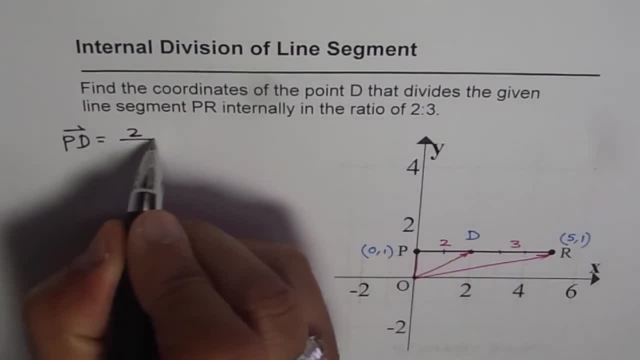 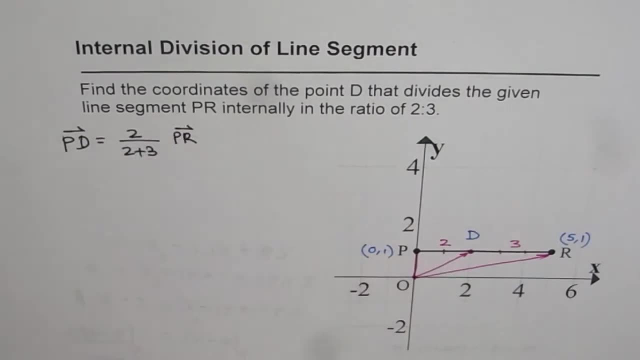 So PD is 2 over 2 plus 3 of PR, of PR, right, So that is what PD is, So I'm purposely not adding them for now. Okay, Now, so we get some relation between PD and PR. We need the relation between OD, OP and OR. 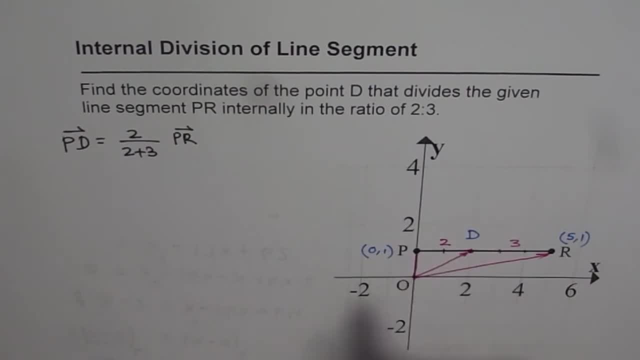 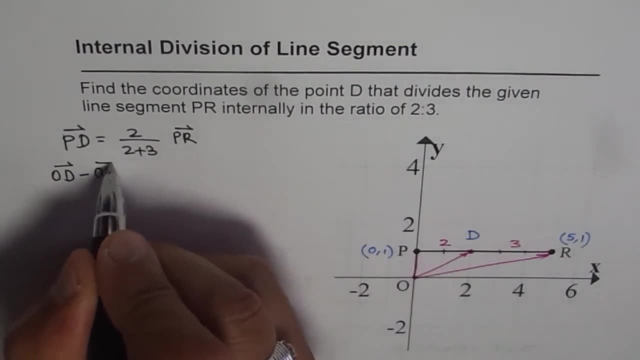 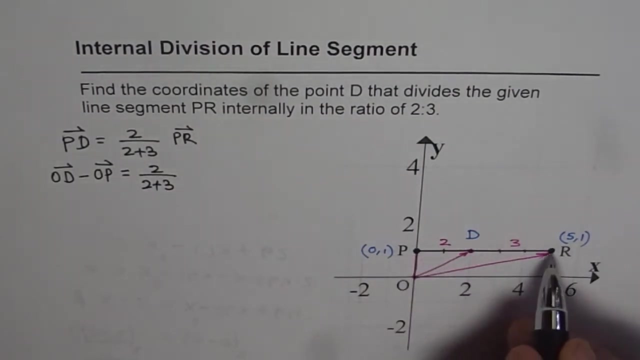 So PD can be written as OD minus OP. So let's do that. So OD minus OP equals to 2 over. Let me write 2 over 2.. Okay, Let me write 2 plus 3. still, PR will be OR minus OP. 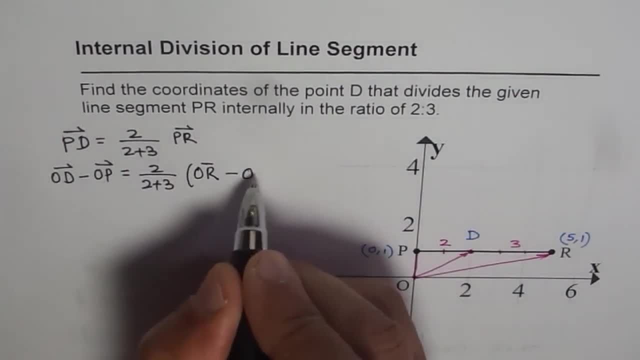 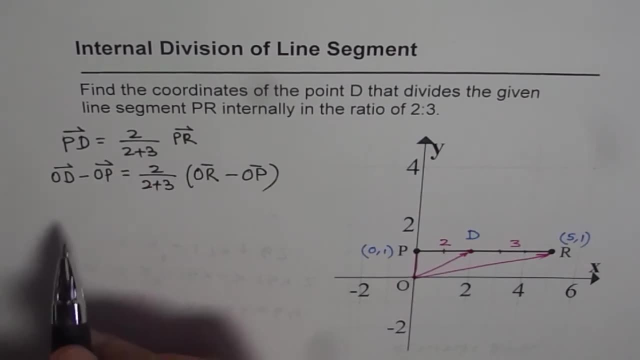 So OR minus OP. So from here we can isolate OD and get the value of OD, So we get OD equals 2.. Let's take OP on this side, So we have 2 over 2 plus 3.. OR Let me write OP first. 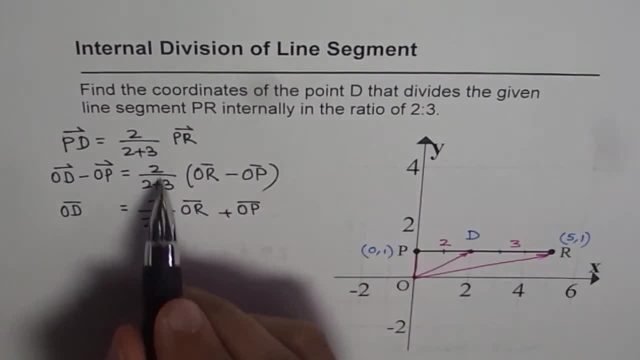 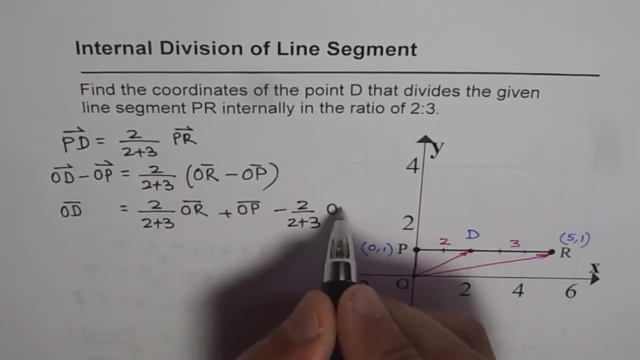 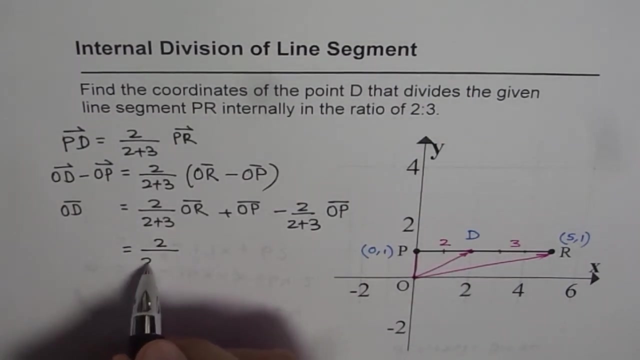 Plus OP, And then minus 2 over 2 plus 3.. OP, Now, from here we know what: OR is 2 over 2 plus 3, OR That's the first term, And here we get: 2 plus 3 is 5.. 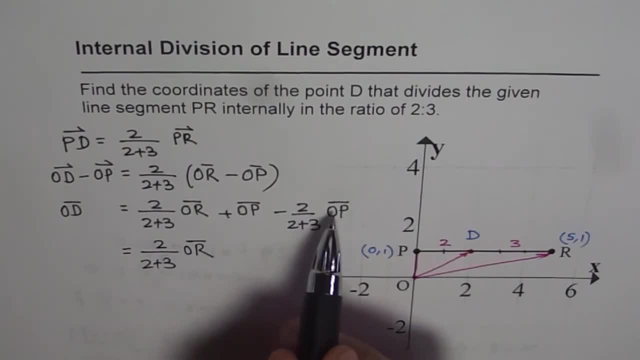 So 5 OP minus 2 OP will give me 3 OP, right. So I'll get plus 3 over 2 plus 3 OP. So that is how I get the value of OD. So I know vector OD is 2 fifth of OR plus 3 fifth of OP. 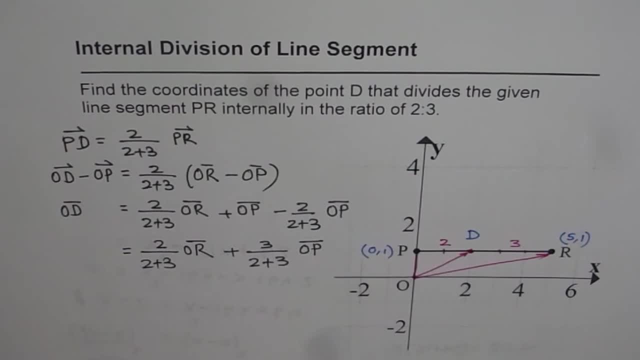 And this 2 plus 3, is the ratio. 2 is to 3.. Correct, So, in general, if I would have had this question, as in the ratio of, instead of 2 over 3, if I replace this with M is to N. 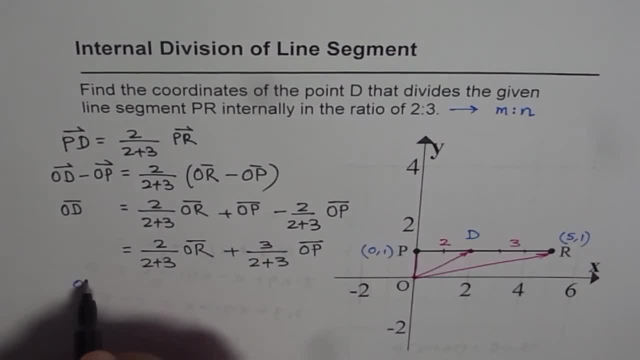 in that case I can generalize my formula right. I can get OD equals 2.. 2 is M for me, So it is M over M plus N OR Plus 3 is N, So N over M plus N OP. 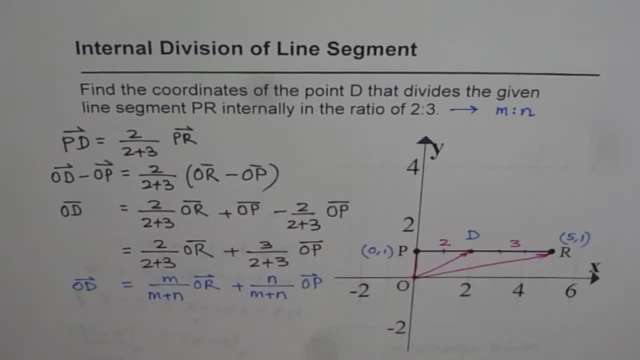 Do you appreciate that? So basically, if the question would have been any ratio, we could have found a relation right Now. since OD is our position vector, we know the coordinates of D, So coordinates of D will be We can find from the given coordinates of P and R, correct? 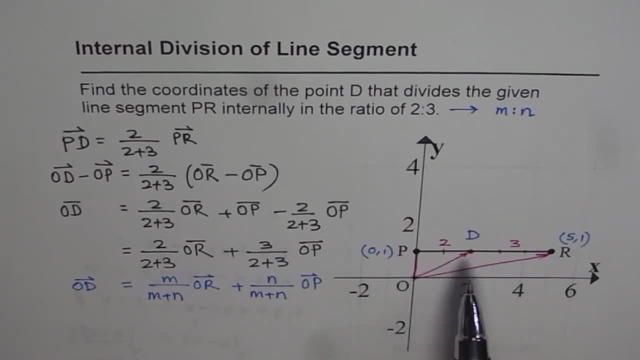 So that's how we can do it. Now let's solve for this particular question. now We know what is OP. OP is 0, 1.. And OR is 5, 1.. Right, So getting back to the question, 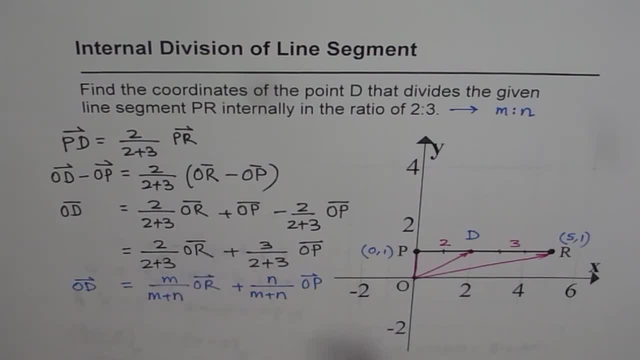 That is to say, let me now- I gave you a general formula, But now let me get back from here, right, So we'll find, So we'll find OD Solve the question now. Okay, But I think you got the concept. 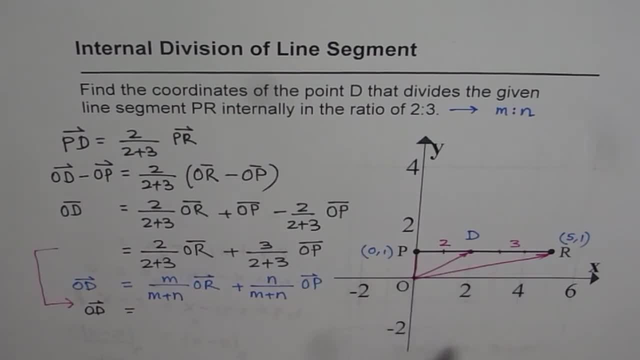 It's not very difficult. We can always find D for any general line using this formula. That is kind of important, right? So we get 2 over 5.. Let me now write down, Since we know it's 2 is to 3 ratio. 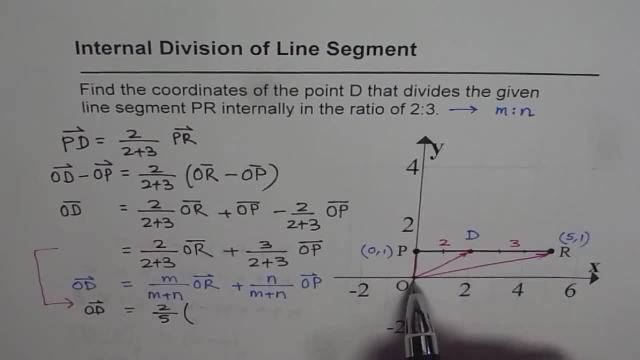 2 over 5 of OR, So OR is 5, 1. Right, Plus N is 3 for me, So 3 over 5 of OP, which is 0, 1. Right. So let's add these vectors. 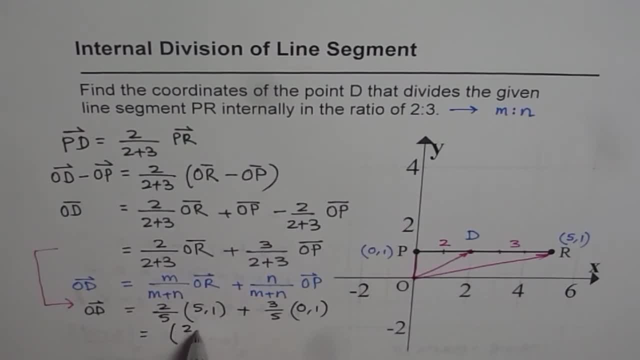 So 2 over 5 gives me just the number 2.. And then this is 2 over 5. Plus 0. 3 over 5.. Correct Now. So let's combine them, Since I'm running out of space.